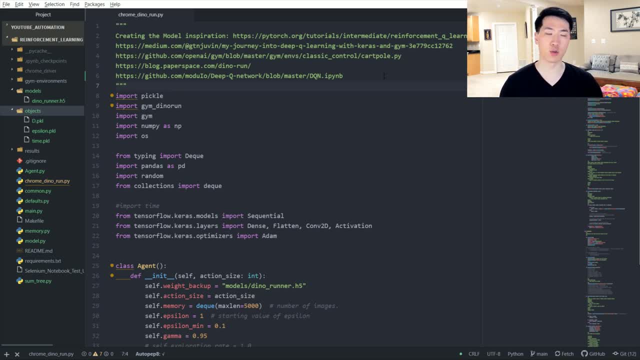 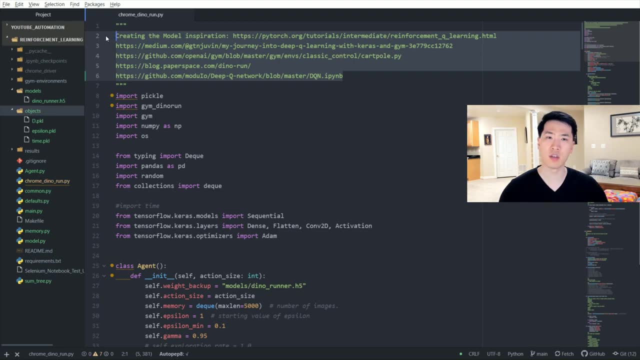 learning process related to the AI Dinosaur game. Note that these links that I attached with this particular script provided a lot of inspiration and a lot of details that I actually used throughout this entire script over here, so do make sure to check them out. 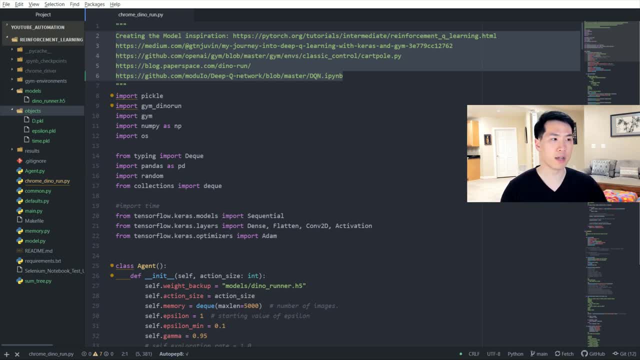 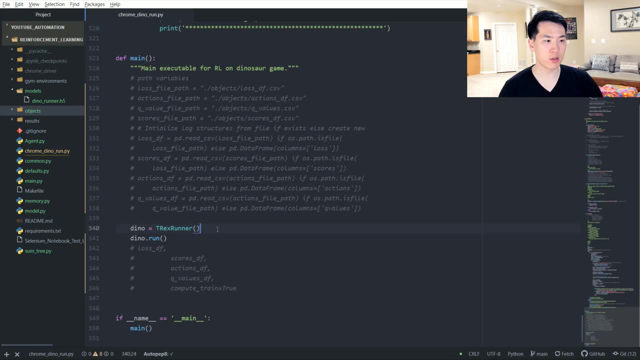 These links will still be attached to the script when I push all of my changes to my GitHub repository, which is attached down into the description. Now let's go over the main functions and the dataframes I've just mentioned. I will actually just go over them quickly. 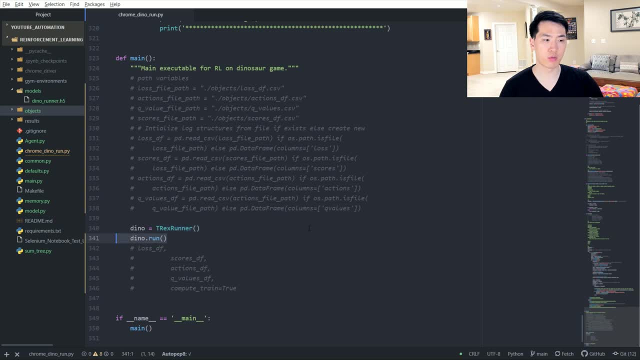 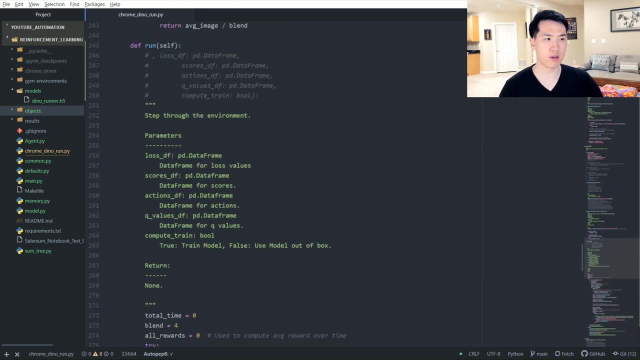 so the only thing I'm really doing here is that I'm just initializing my T-Rex environment in this case, and then I'm calling the run function. Note that all these other variables that I've just commented out are related to just recording each one of the given, I guess like loss scores. 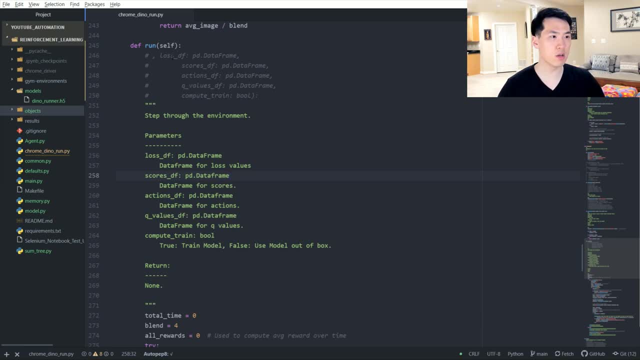 actions or cue values, but I did not really I didn't actually implement it but due to the complexity. But you could do so by just passing in the dataframes, a part of the function and just those to its associated data frame, and you can have somewhat of a logging structure related to. 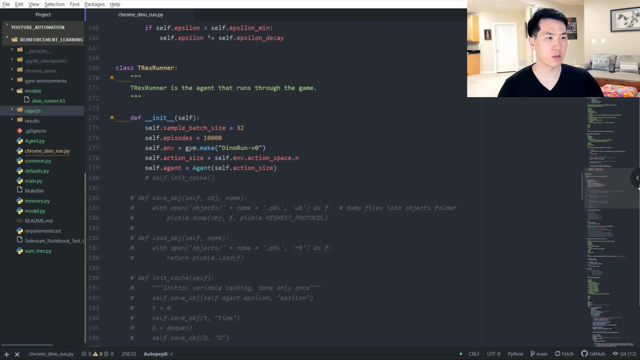 your data frames. before we go to the run function, let's go ahead and go over the initialization part. so this is just the batch size related to however many images that we want to extract from the overall memory array that we have going on, and this is we're just going to be calling out. 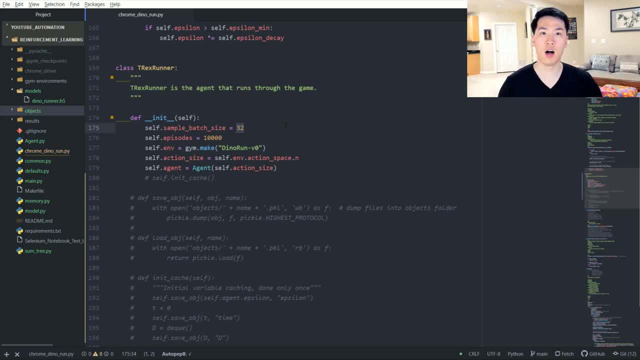 32 random images and we're going to be training the predictive network and, you know, update its weights. we have 10 000 games over here where each game is. this is also in sequential order, so it's like with each game being the dinosaur starting and then it ending on some obstacle because it 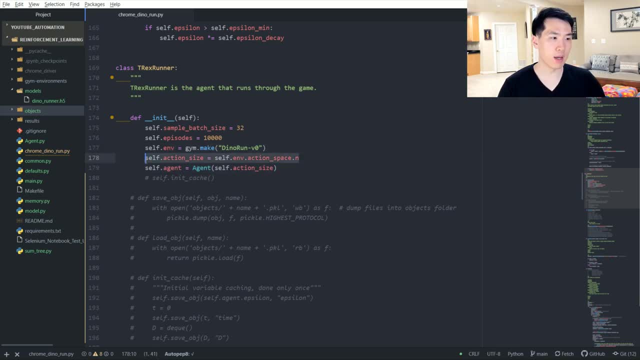 failed the game. we initialize our environment- we have our action size- and then we initialize our agents where our agent is essentially our dqn model- our action size is our dqn model- and then we initialize our agent where our agent is essentially our action size. and then we initialize our agent where our agent is essentially our dqn model. 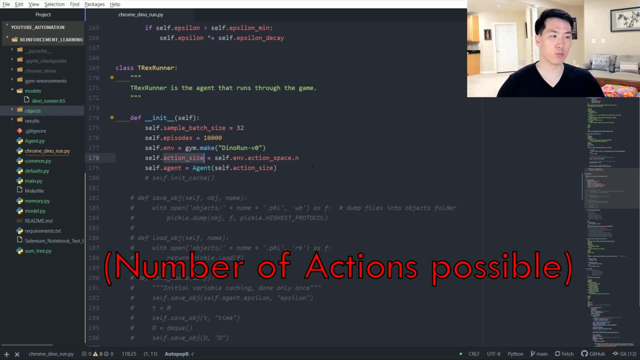 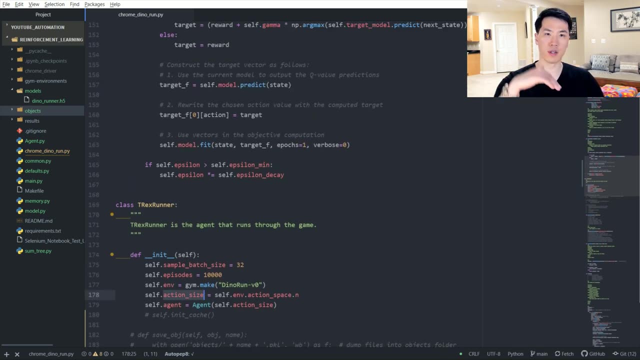 action size is two. uh, it's gonna be initialized. uh, well, you're gonna be calling it zero or a one, depending on what action is going to be, where zero is doing nothing and a one is where the dinosaur is actually jumping over the obstacles. so let's go over the agent really quick. this is the agent. 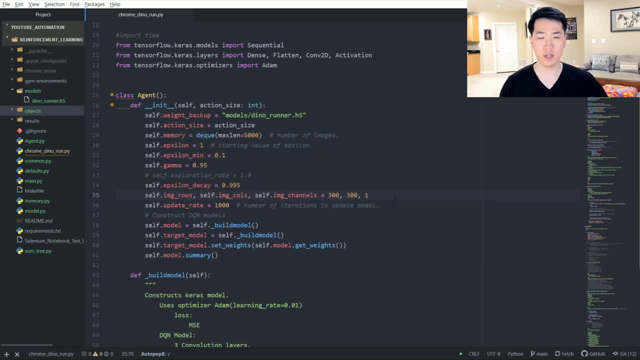 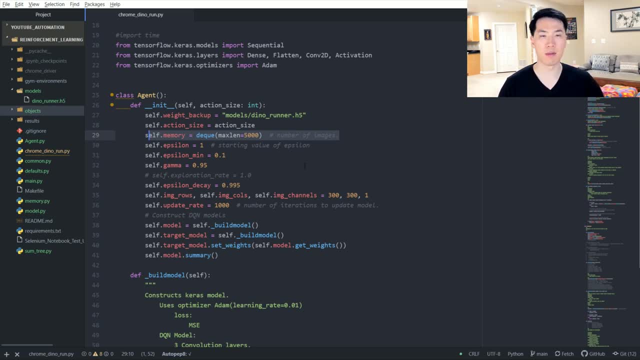 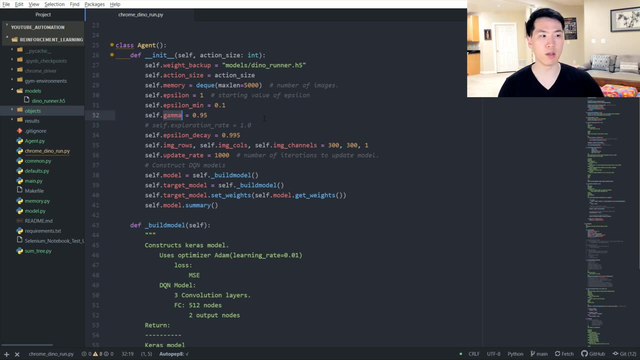 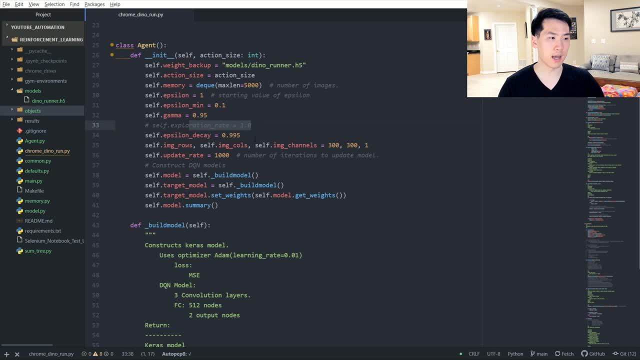 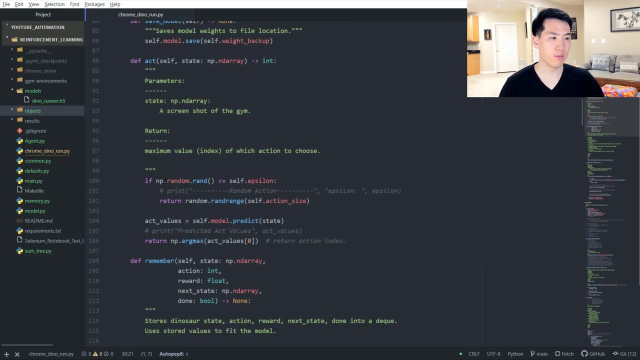 update the q values. we also have our decay over here, so the epsilons are pretty much just used to update or decide whether or not we should be using a random value right here to, you know, predict what the dinosaur should be doing or should it rather go ahead and, you know, utilize the actual model and 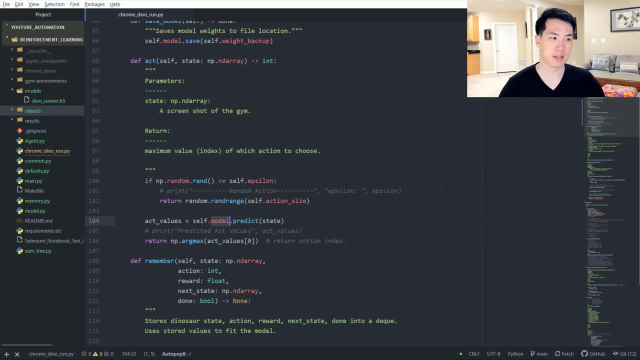 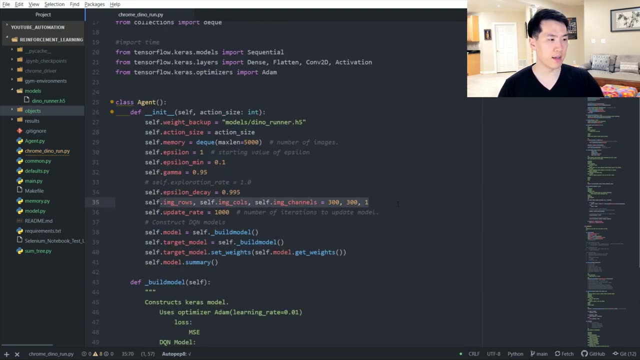 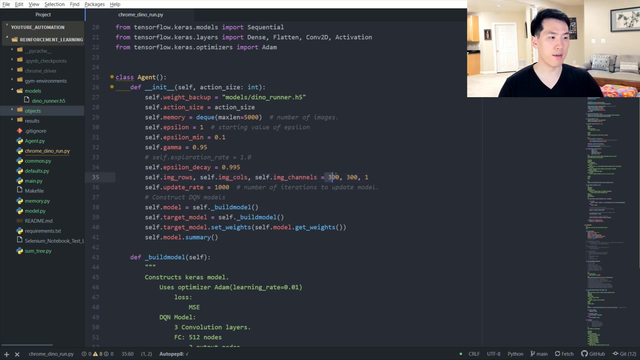 itself and predict based on what state is currently at. but we use that epsilon value to determine if it should just use random actions or so, okay, so after that we have our dimensions of our given image, in this case 300, 300 by one, where one is the number of channels, and then this is just the rows. 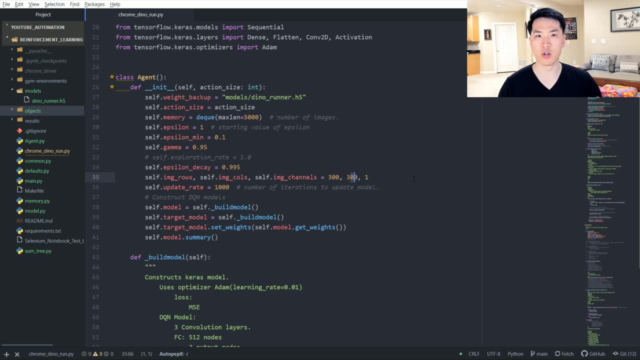 and this is the height. so it really depends on, uh, how large your dimensions of your specific image you would want it to be, but in this case i just made it, so that's 300, 300 by one. we have, of course, our update rate, and this is for every 1000 iterations where we want to update the weights. 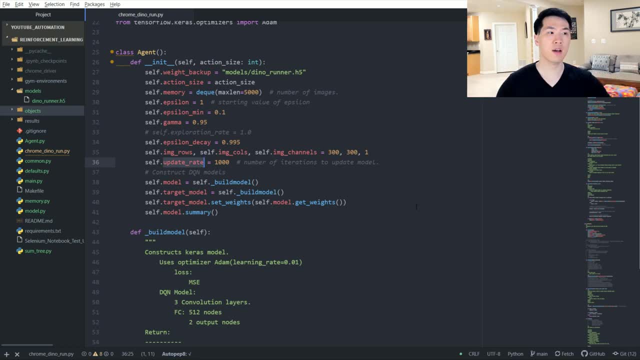 of our predictive network to our target network. so our predictive network is the one that's continuously being trained right and it's like slowly diverging from the original model, which is just, uh, right here, our model portion, right here now. actually, no, it's going to be our target model. 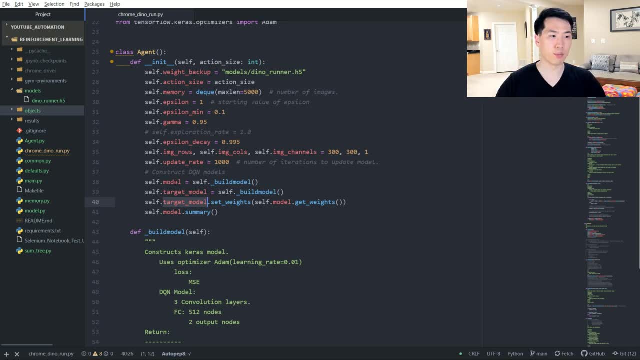 i should say our target model is our original model and our predictive model is just our model in this case. so the primary reason behind this is that it's just the dqn process of where it has like two neural network models. it's training one and then updating the old one, um, after you know, after in this case. 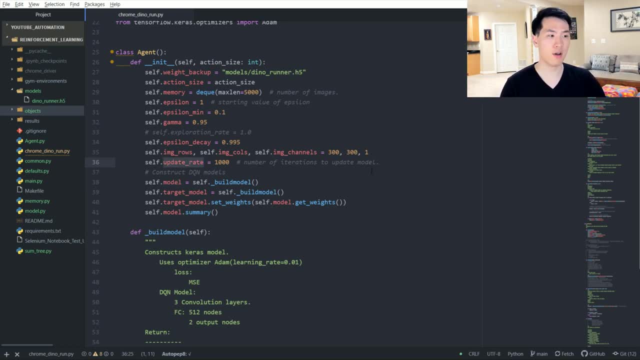 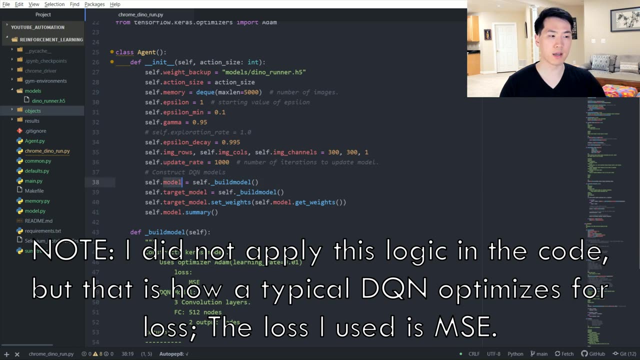 1000 iterations for the update rate here. uh, and primary reason behind this is to somewhat keep the models in check, and you're gonna have two different q values, based on the predictive model and the target model itself, and then the loss function will be, you know, subtraction of those two and 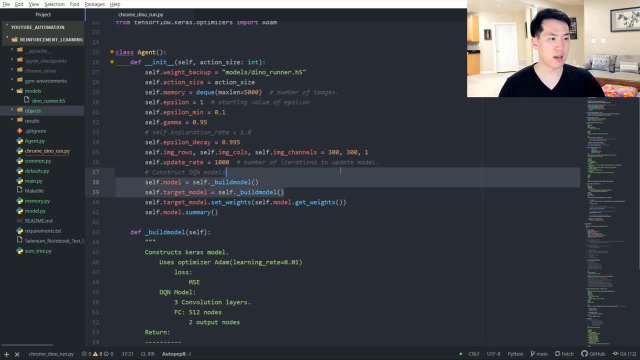 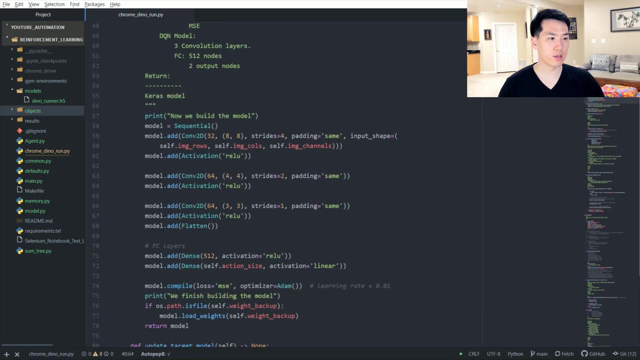 values. that is going to be the loss, nonetheless. after that, after you initialize the values and update its weight. i just print out the summary over here. so what the model looks like over here is that we're just- i'm using a charis, by the way, charis backend, but it's gonna be three. 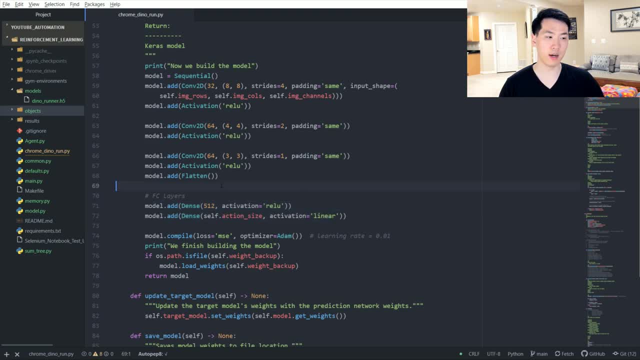 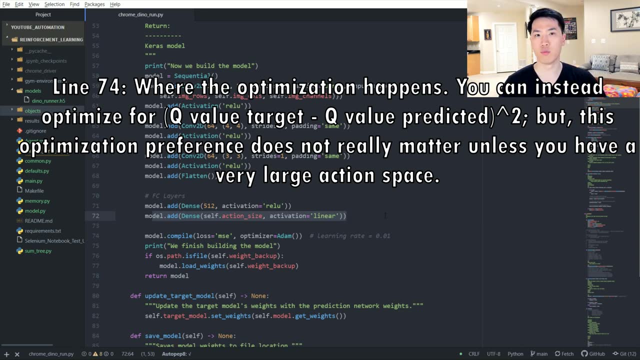 convolutional layers and connected with a fully connected layer of 512, and then go ahead and create the number of outputs with whichever number of actions you're going to be using. in this case i have two, so it's gonna be ending with two output output nodes, i should say. 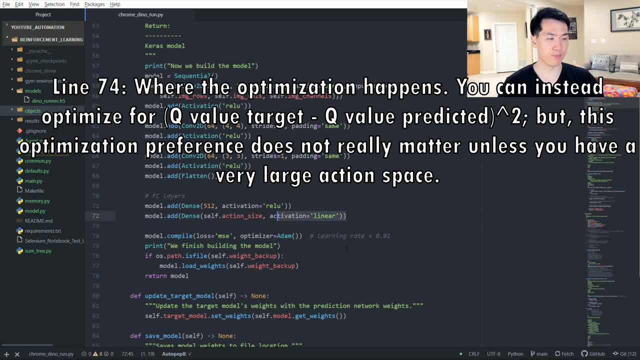 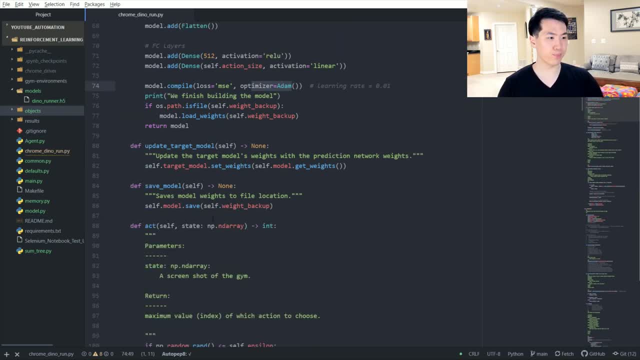 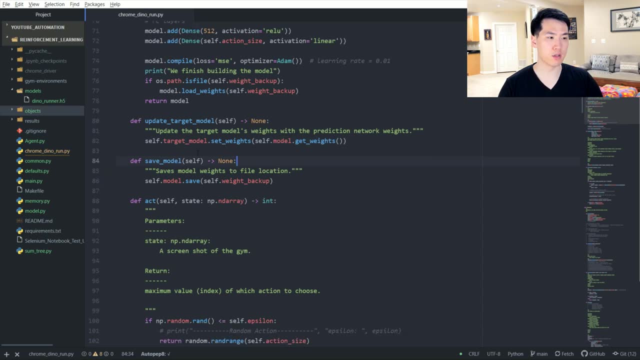 based on doing nothing or jumping, and then just activating linear and, of course, use the atom optimizer, and then you have your model and then the other functions are just, you know, update the target model based on the weights, based on the predictive model weights, i should say you have. 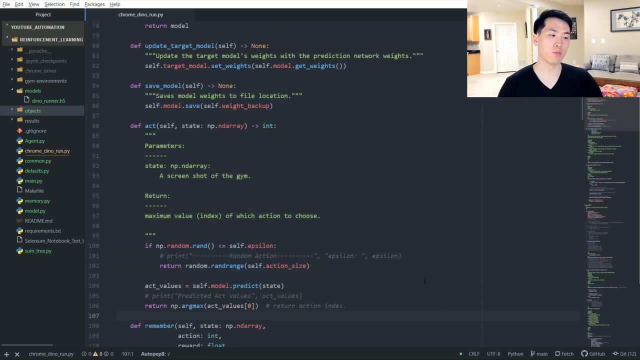 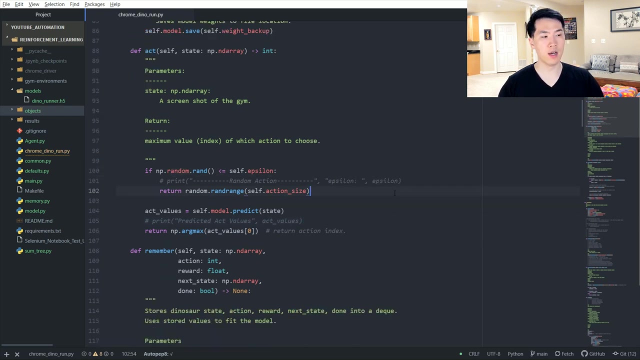 a safe model function. and then this is our act function, which is, as i mentioned earlier, this determines whether or not the dinosaurs can be, you know, jumping or doing nothing based on a zero or a one value. and that's what these logics are doing over here, where it's using the epsilon to determine whether or not it's. 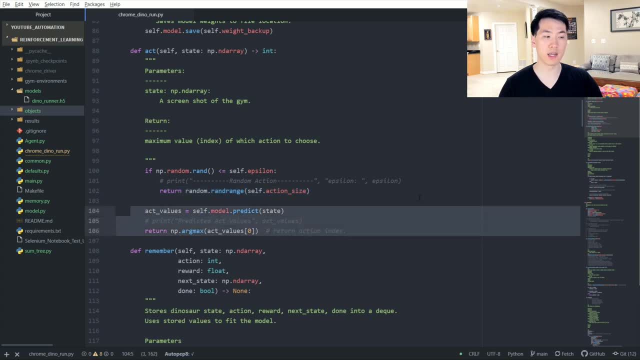 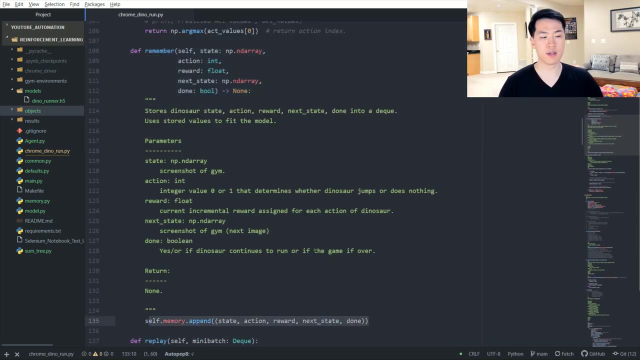 going to be using a random state or a predictive state either, or is going to have one of those values, and then we have a remember function. then this is just appending images and its associated action reward: next date and done. we'll go a little bit deeper into this. 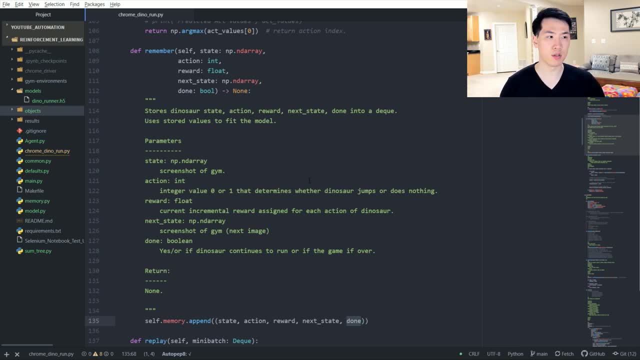 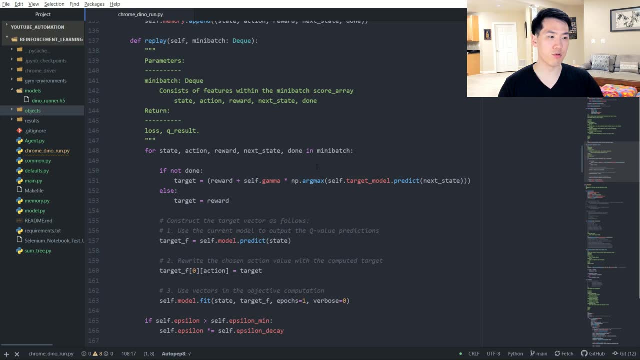 but this is what the deck of 5000 images are going to be appended by using this function over here and then our replay. this is just going to be going through our given memory based on this member over here. it's just going to be iterating through the memory and it's going to be in batch. 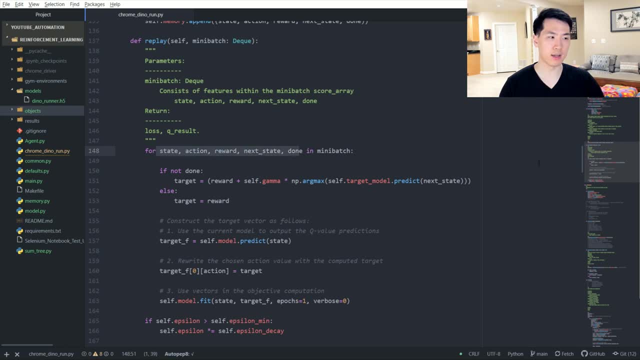 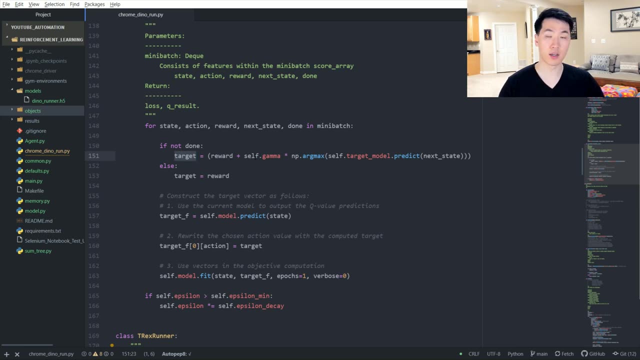 sizes of 32 images, based on the state action reward and next state done, etc. and then it will decide, you know, whether or not it's going to be updated in target queue value or just be using the regular q value. if it's not done or done, and then you know, just go through the process. 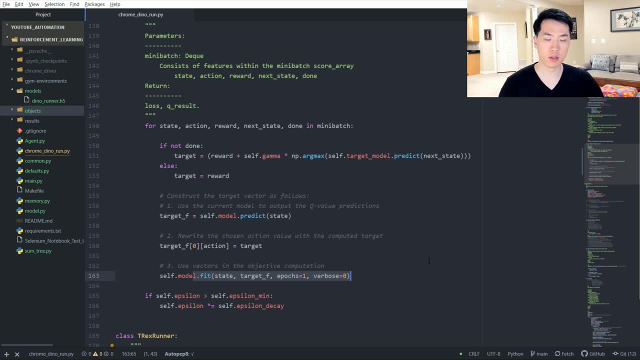 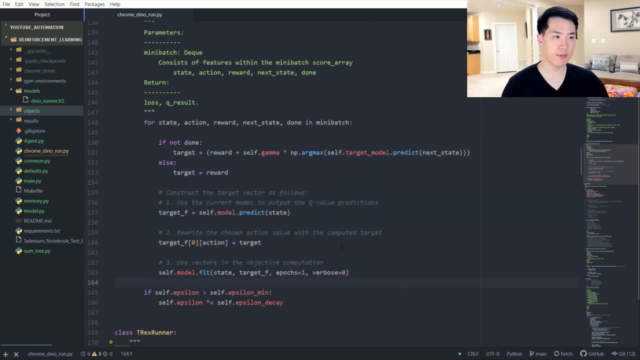 over here of where it's going to be iteratively training its model based on the predictive network model. okay, and then once the model has been fit and everything like, once it's done, iterating through the mini batch, we will then update the epsilon value if it's greater than our epsilon. 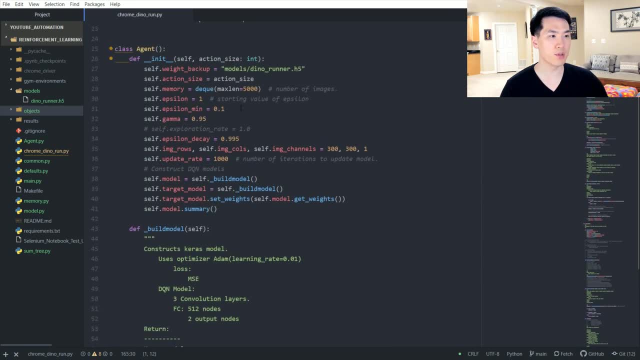 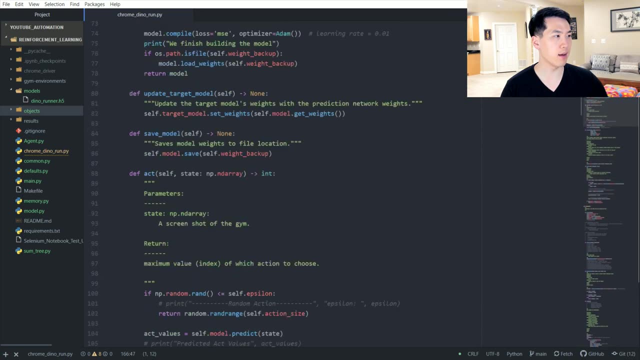 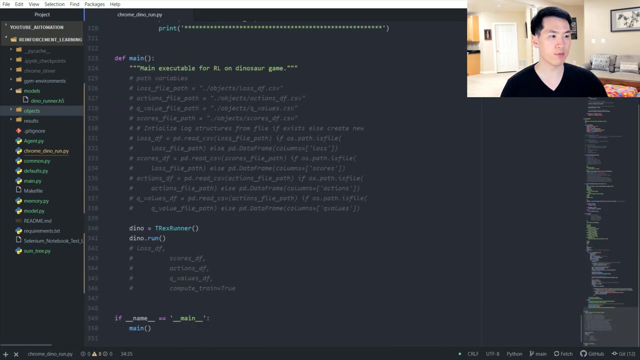 minimum, which in this case the epsilon minimum, was a value of 0.1 over here. so if it's greater than 0.1, it will go ahead and decay the epsilon by multiplying by the epsilon decay, which is 99.5, as noted there. okay, so let's go to the run function. um, that is essentially underneath the 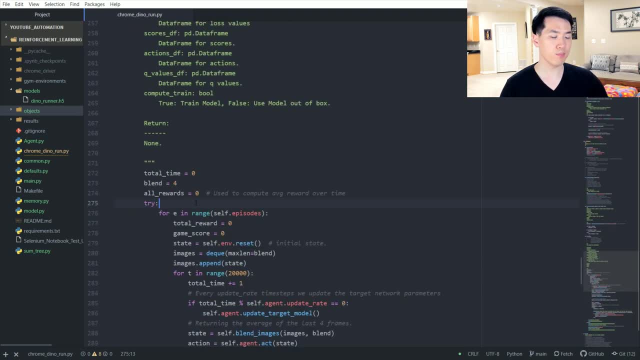 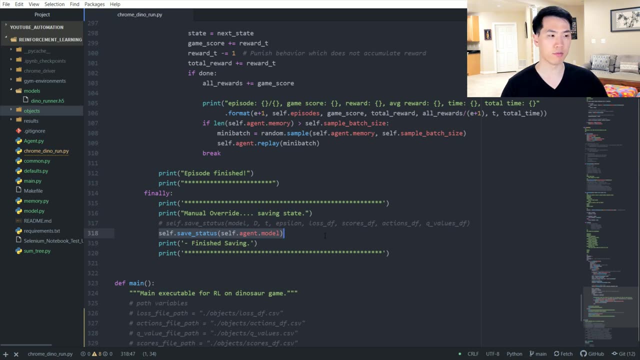 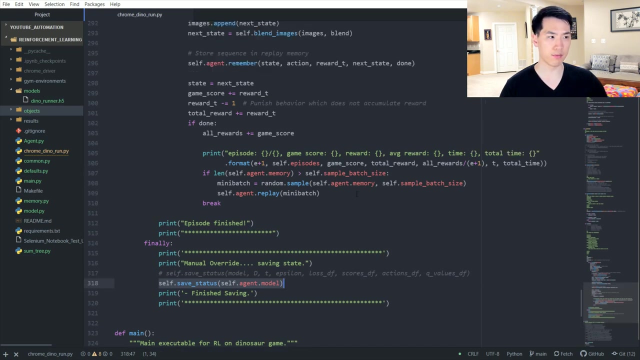 dyno initialization part and it's over here and so very high level. i have a try finally, uh, statement going on. so if i want to manually get out of this particular program, it will save the model. inside of the model is dino runner dot h5 file and i will automatically have the most up-to-date model. 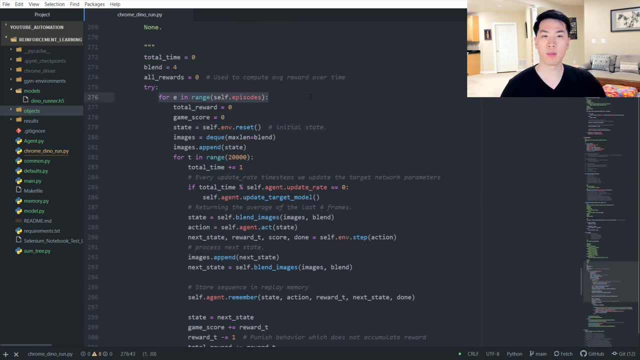 uh, if i want to exit out this particular program, all right, so we'll be iterating through 10 000 games over here and then we have total reward game score. these are going to just for, like you know, um understanding purposes, on our given output for our print statements. uh, we're gonna have. 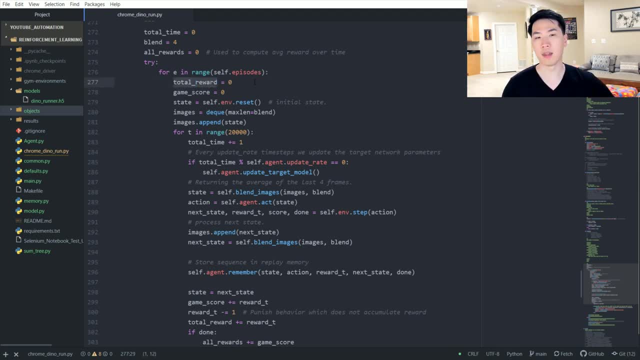 you know, a decimal value or so if the dinosaur is continuing on his way, uh, as a increment of 0.1, or if he loses, you know, those could be a decrement of one, uh, so we're gonna have like a positive or negative value reward system going on here. we're also having to have 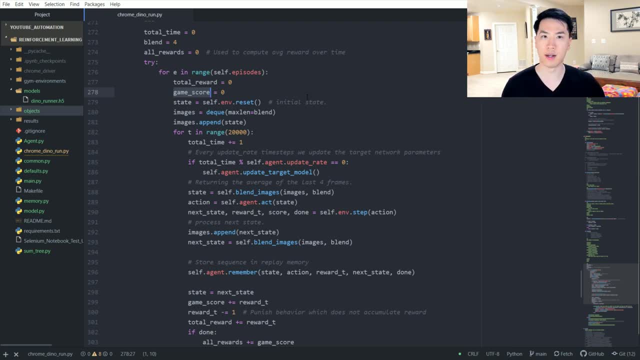 a game score pretty much to determine you know how far the dinosaur has traveled. now, at the very beginning of each game, we'll be resetting our environment so that we're at the very beginning of the game. that's pretty much what that is happening here now. this is very important, uh, we. 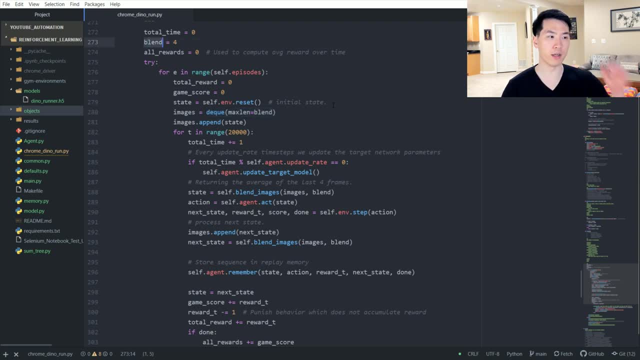 have a deck of a length four, determined by blend over here, um, and i'm just gonna be appending the states to this deck. now, primarily, what this uh deck is going to be doing is that it's going to be an amalgamation of four images, specifically using 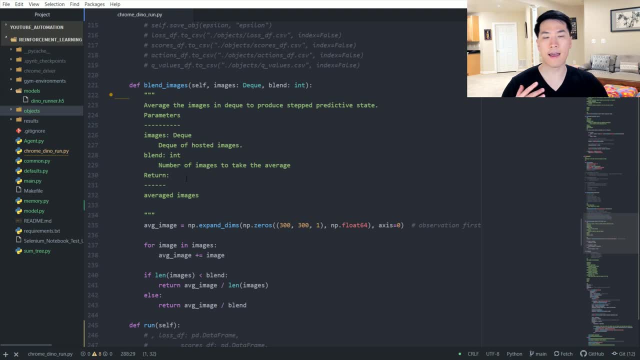 this blend images function, which is essentially just taking the average of all the pixels that exist within that deck. if there's less than four values or four pictures, i should say, we do take that into consideration and we just take the average of whatever else is in there. so that's. 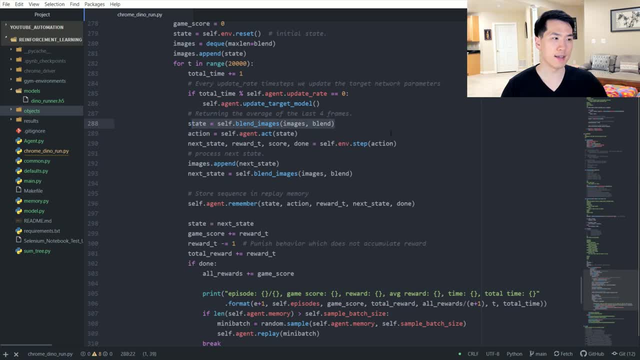 pretty much happening there. the reason behind that is that it's going to get pretty much just four frames all together and then you know, uh, to generate some form of a predictive outcome for the next state, uh, and then we'll be plugging in that predictive state into the action function to retrieve some form of an action. 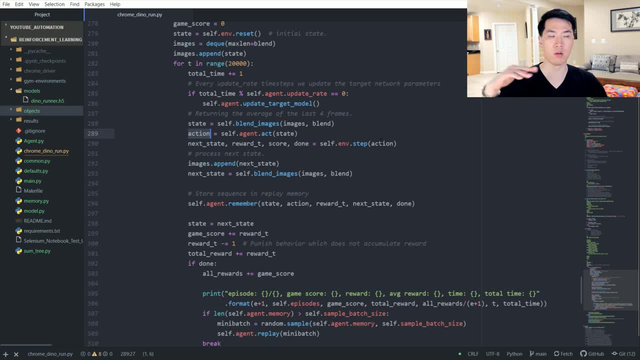 whether or not the dinosaur should be jumping or you know, doing nothing essentially. so we plug in that action to the step function over here and then we get four additional values. uh, we'll be the next image that comes along. the associated reward with that, with the previous action that we 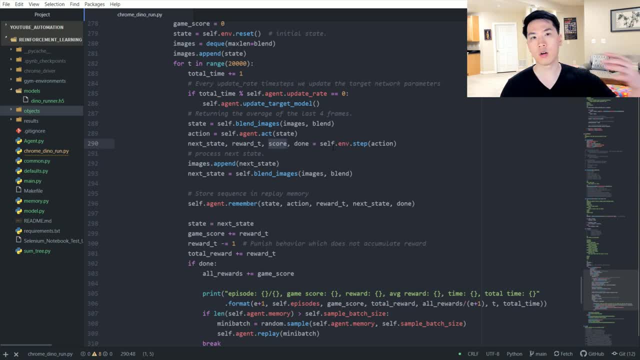 have already taken, uh, the associated score. you know how well uh the uh dinosaur has done so far? you know? just get the the roadmap score and how much distance has the dinosaur traveled and whether or not the dinosaur has actually hit an obstacle. um, and then we'll just be. 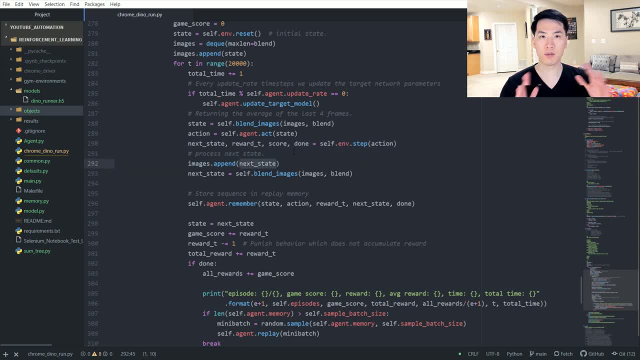 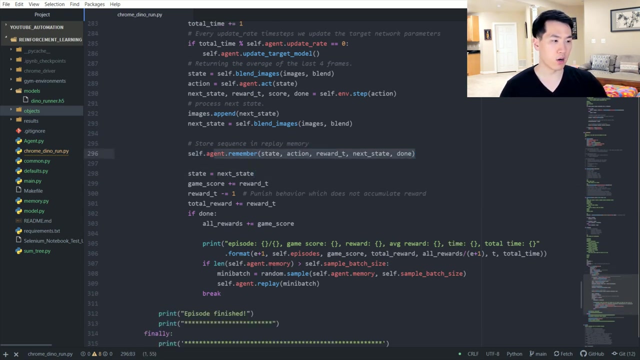 appending that, uh, that new image to the image, uh, deck, and then we're gonna do another blending sessions, um, to get the next appropriate measure. we're then gonna be plugging that into our memory buffer over here, um, and this is where, uh, we are actually going to be, uh, mini batching from. so we'll 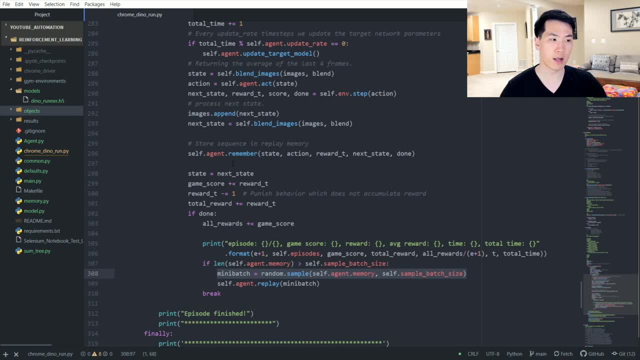 be sampling 32 images, or i should say 32 values, from the array that this, remember, function is appending to and of course we have, you know, some additional reward systems. are, you know, incrementing or decrementing, and the old state becomes a new state and it keeps iterating through. once this for loop has run, 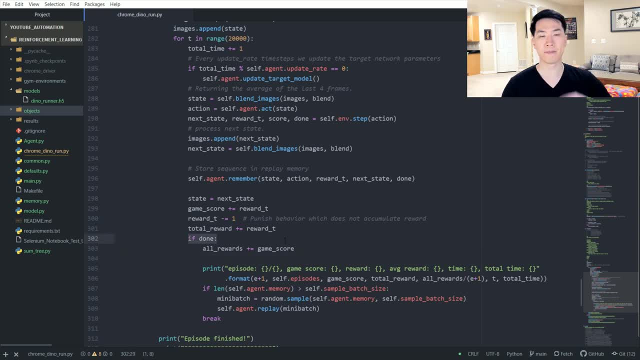 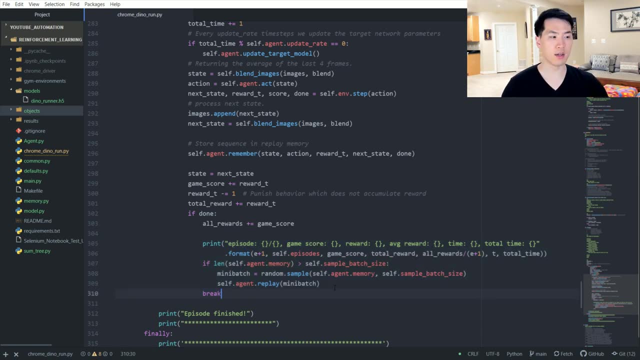 its course and, of course, if the dinosaur has crashed, we'll then want to train, based on his previous experiences, and hopefully we can get all of the, all the failures and successes based on that one game in order to, you know, hopefully improve upon, you know, its own understanding of how the game operates. so let's do a really quick demo on what 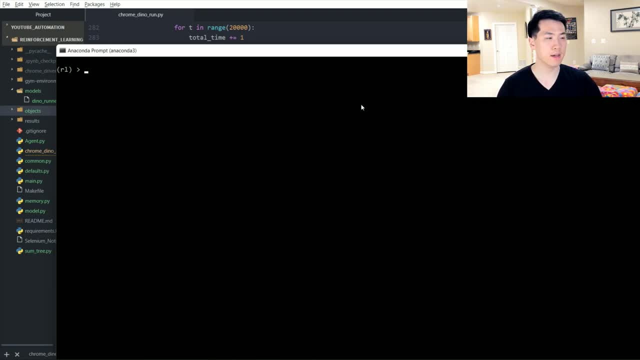 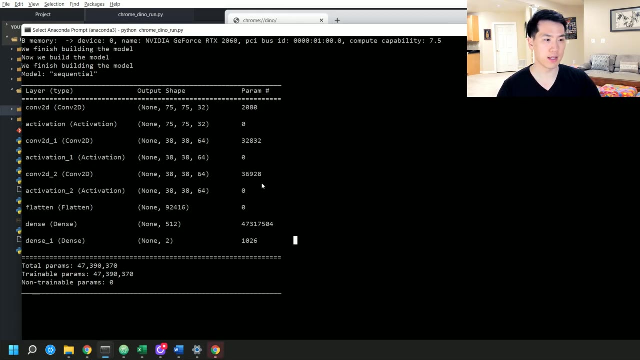 might look like. let's go over here. all you do, just do python, and then chrome dino run. go ahead and run that, and then a selenium web browser just popped up over here. that's good. uh, this is our model. that was initialized. that we printed out using the selfmodel. this is our um. this is our. 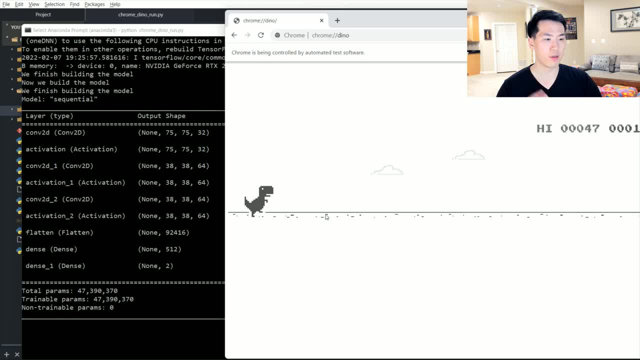 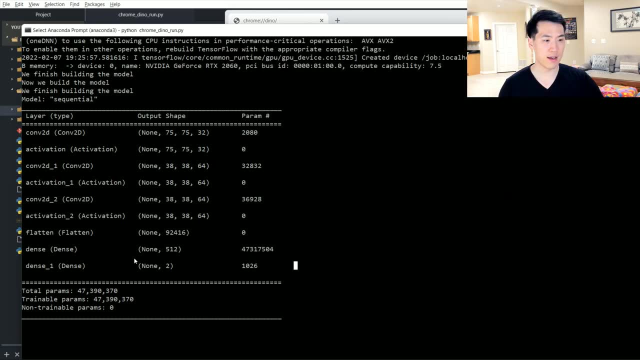 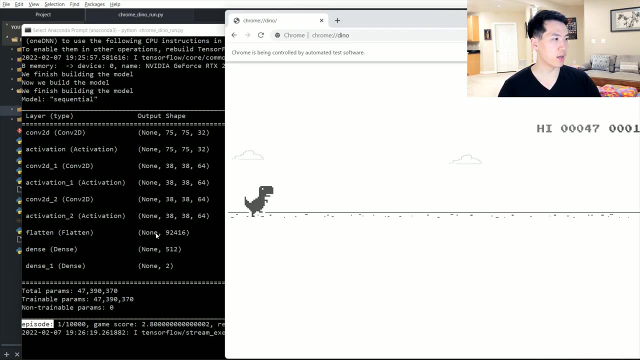 target model and for the very first 100 or so iterations that's going to be going through, it'll, you know, like hang up on this. however, within each of the episodes i'll be going through, it will become more streamlined as time goes on. so this is pretty much my demonstration on the reinforcement. 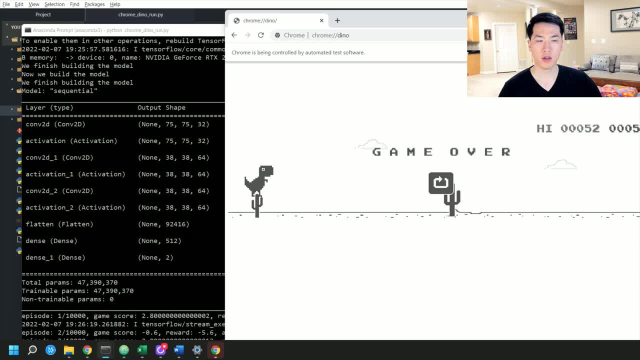 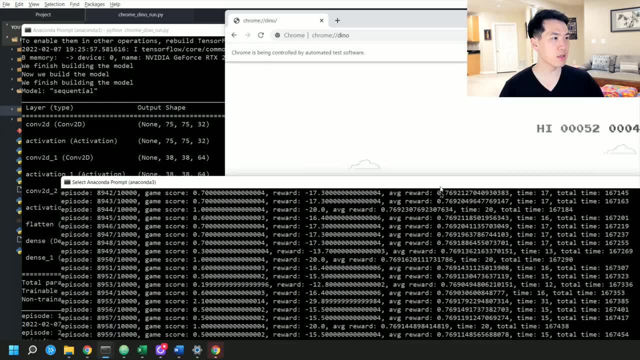 learning aspects of the dinosaur games and after about 9 000 or so iterations that i ran through. the highest score i actually got from this reinforcement learning process of this dinosaur doing its thing was about 150.. there are definitely a few ways that this process can be. 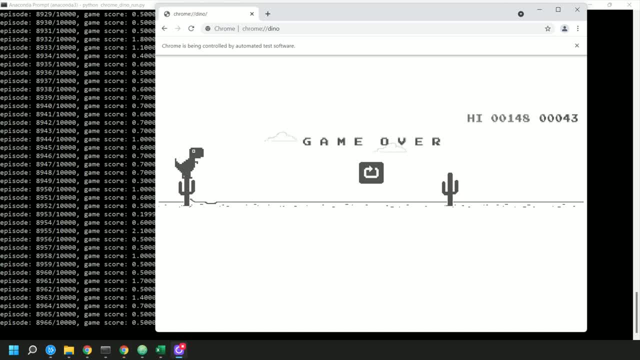 improved. first i can use an entirely different deep q model, such as a sarsa model or a or a double deep q model. for that instance, i can also switch up the policies that determine which action the model decides to use initially. this particular policy i was using was a epsilon greedy model and 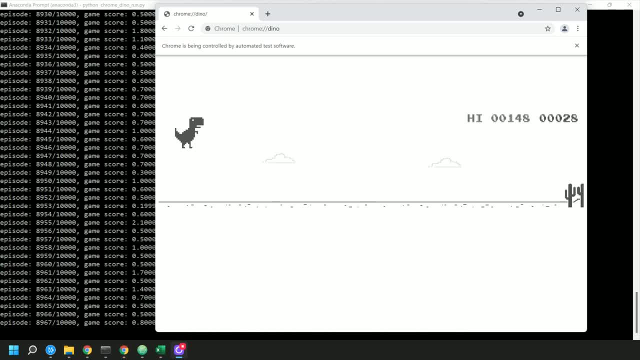 this policy can change. furthermore, i can also adjust how frequent the prediction network updates the target network weights for faster learning and, lastly, to speed up training time. i could also run the selenium web application in parallel to have multiple games running for faster results. nonetheless, i ran this process for